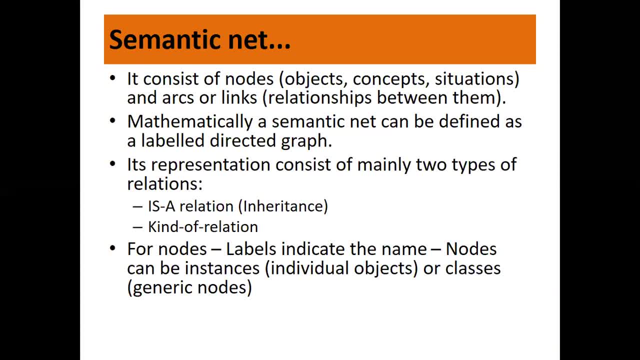 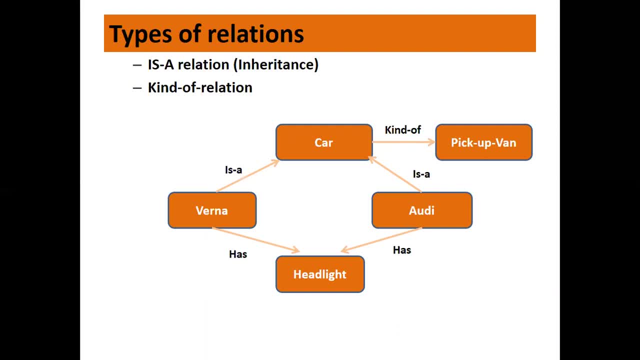 that is an individual object or a class, that is a generic node. Now let us see how the relations are shown. So you have two relations. that is is a relation and kind of relation If you look at it now. So you have two relations. that is is a relation and kind of relation If you look at it now. 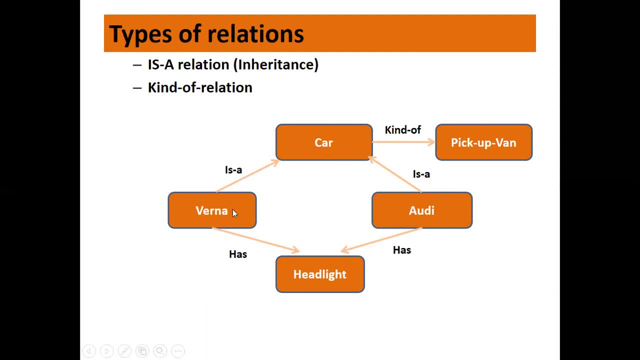 So you have two relations. that is is a relation and kind of relation. If you look at it now, Varna and Audi are is a car. Varna is a car, Audi is also a car. So if you look at carefully, Varna and Audi are instances of the class car. Right Now, Varna has headlight Audi. 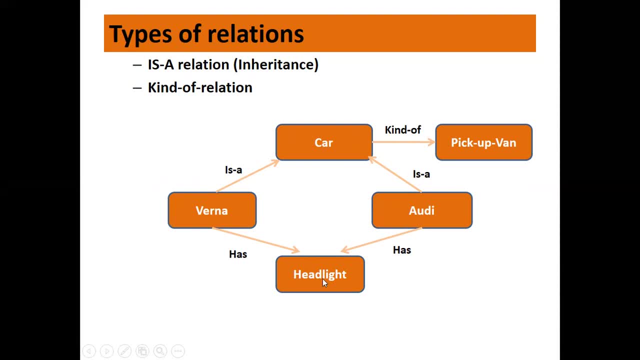 also has headlight, Is it fine? These are the attributes. we can say: Varna has headlight and Audi has headlight. Varna is a car and Audi is a car. Now, any car has a headlight. Any car is nothing, but it's a kind of pickup van. Car is nothing but a kind of pickup van. 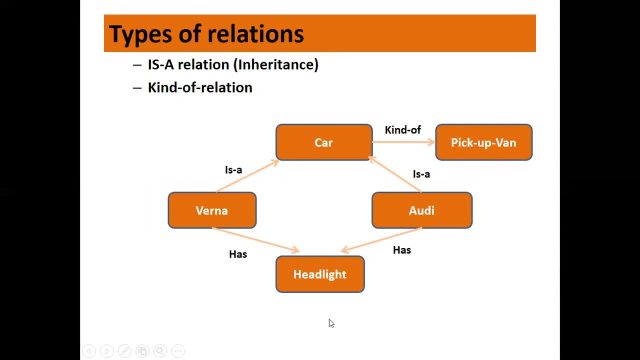 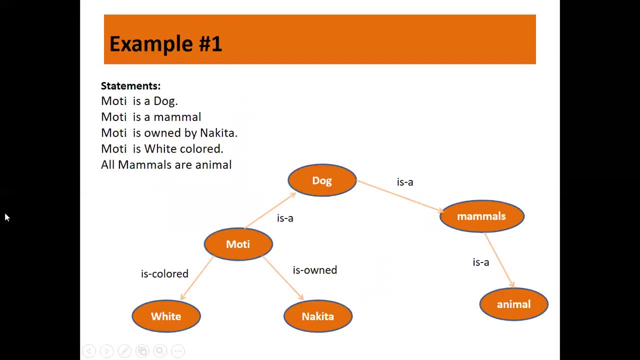 Is it fine? It's very simple. You can represent real life entities or situations Right Now. let us look at an example Now. these are the statements given and you need to represent it in a knowledge base using your semantic net. What is the statement? You have a dog. 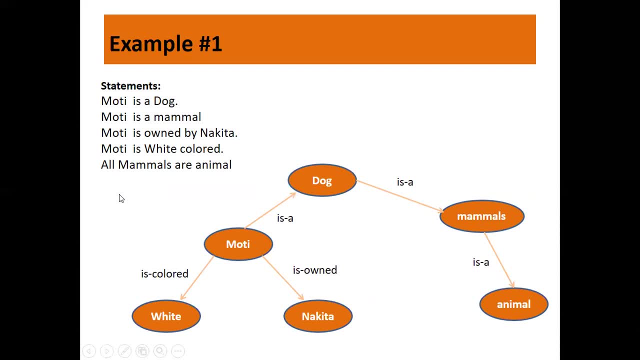 called Moti. Moti is a dog. Moti is a mammal. Moti is only a dog. Moti is a animal. Moti is owned by Nakita. Moti is white in color and all mammals are animals. Right Now, we 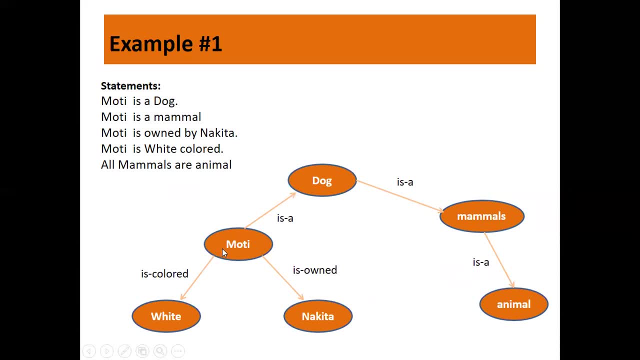 start with the main entity, that is, Moti. Moti is a dog. Moti is colored white. Moti is owned by Nakita. Dog is a type of mammal and all mammals are animals. Is it clear? So such a simple way of representation. 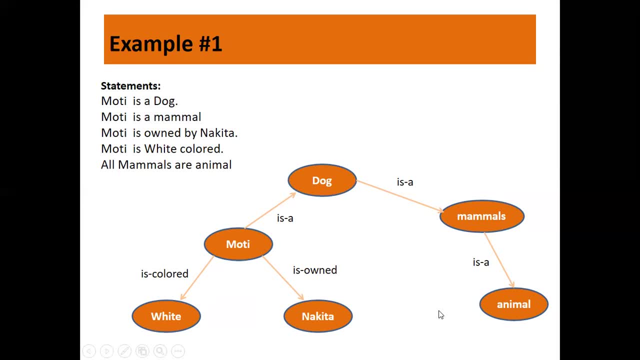 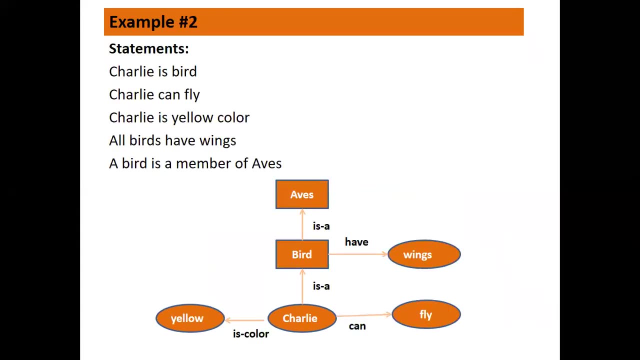 I think this is the easiest thing to understand In knowledge representation semantic net, because our English-like sentences can be represented so easily. Let us look at another example. Now, again here, what we have: Charlie is a bird. Charlie can fly. Charlie is yellow color. All birds have wings. A bird is a member. 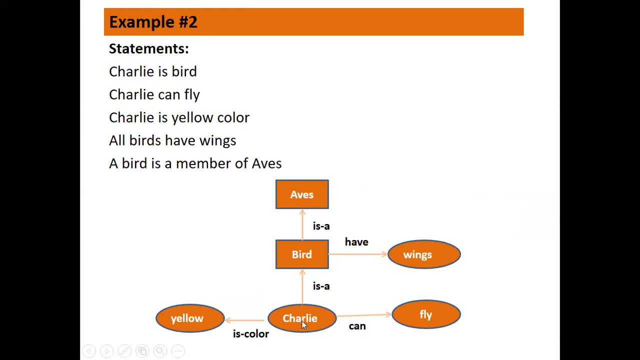 of class Aves. Again the same thing. Charlie is a bird. So you can just think of this, Charlie, as an instance of class Bird. Right Bird is wet, A bird is dry. A bird is dry, right bird is derived from the class is right. so charlie attributes, charlie what attributes? 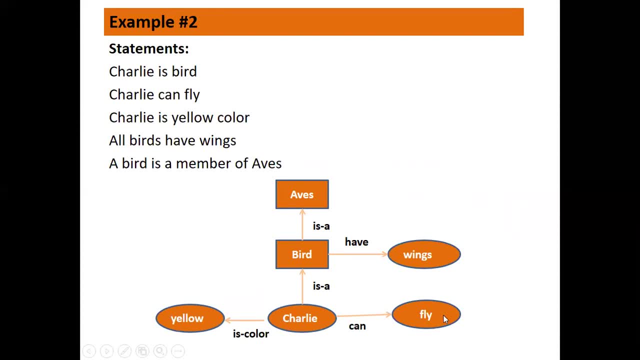 charlie has, charlie is yellow in color and charlie can fly right. if you imagine this as a class, then this is a function and this is a attribute. fine, so charlie is a bird, charlie is yellow color, charlie can fly right. birds have wings. but is a entity of class, is fine. now, if you look at it carefully, 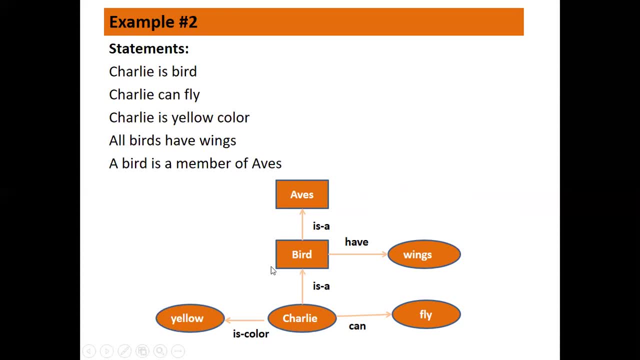 i have put these two in square in the rectangular boxes, but rest are all in a oval shape. why, if you look them carefully, charlie is an instance, but bird is a class. is is a class, right so, but charlie is instance of class bird, so this is a class and this is an instance. the drawback here is in this case. 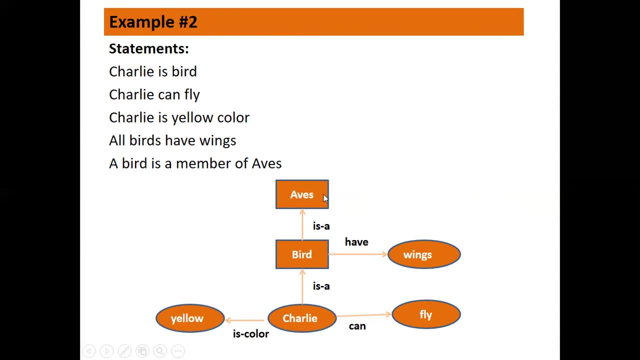 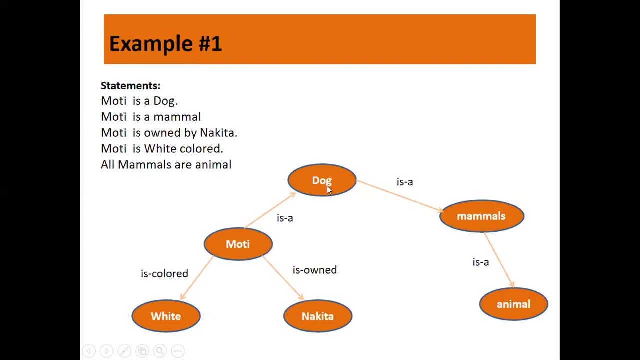 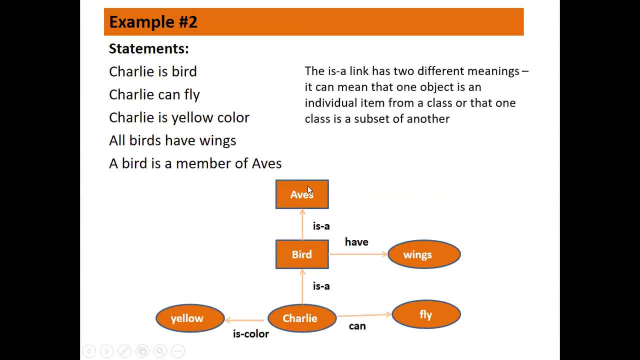 of semantic net. you cannot differentiate when the representation will not help you in differentiating between a class, a subclass and an instance, because all will be represented like this. right now there is a link, is a link you can look at. this easy link has two different meanings. it. 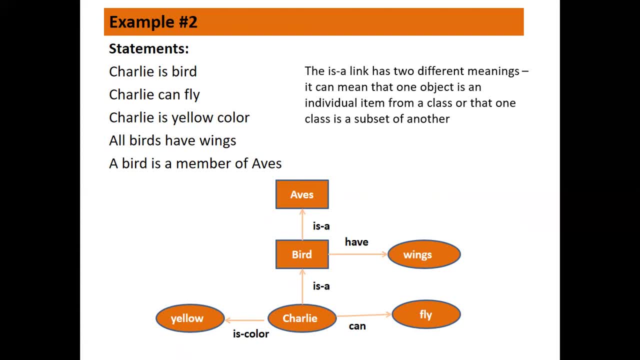 can be an object in an individual item from a class, or that one class is subset of another. now, if you look at charlie, charlie is an, charlie is an object of class. bird and bird is a subclass of class is right, but both are represented using. is a relationship, is it fine? 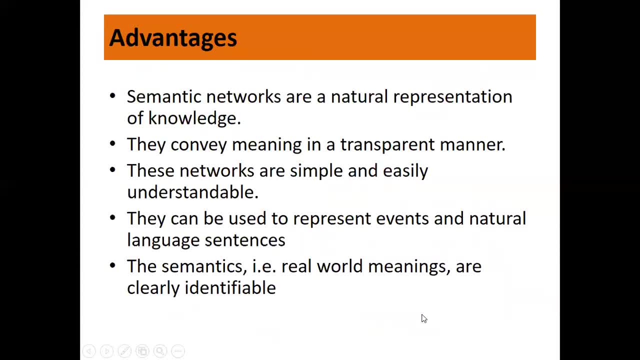 okay, now let us look at the advantages of semantic net. these are natural representation of knowledge, as you have already seen the examples. they convey meaning in a transparent manner, because as soon as you look at the graph, the thing is clear: what it is represented. these networks are simple and easily understandable. they can be used to represent. 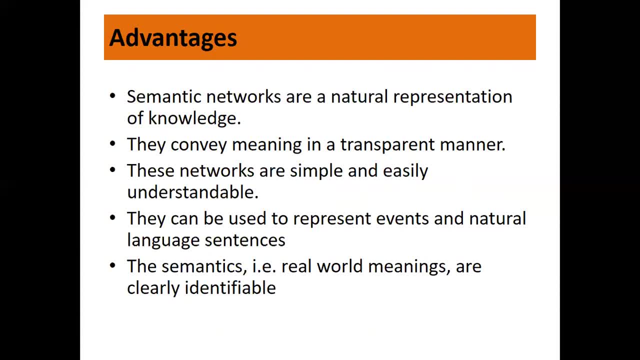 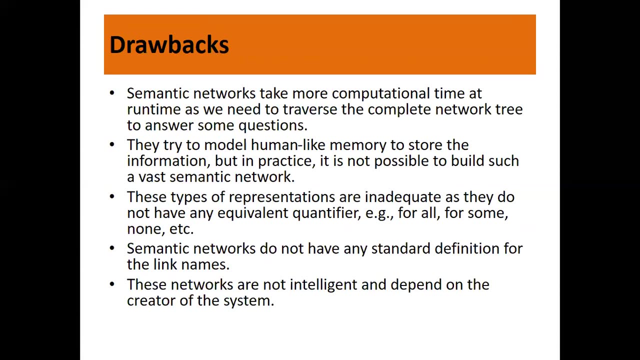 events and natural language sentences, as the example is already given. the semantics, that is, the real world- meanings are clearly identifiable. fine, now let us look at the limitations. semantic networks take more computational time at run time. as we need to take a closer look at semantic networks, they don't travel the complete network tree. to answer some, 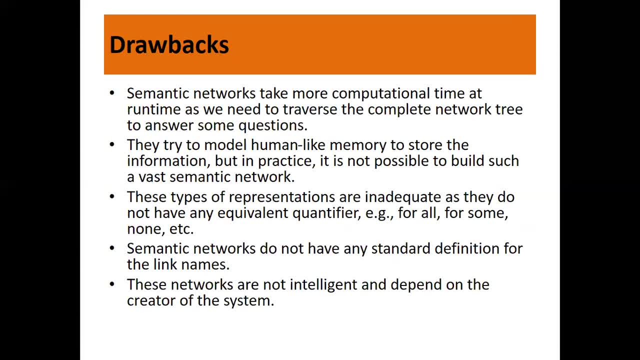 questions. they try to model human-like memory to store the information. human-like memory in the sense how we have neurons and all neurons are connected. the same thing is depicted here, but in practice it is not possible to build such a vast semantic network. these types of representations are inadequate as they do not have any equivalent quantifiers we couldn't represent. 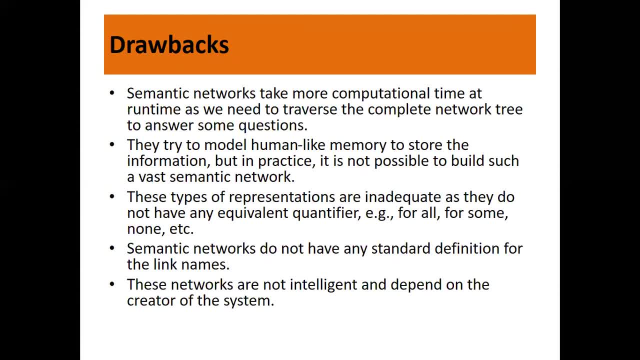 there's no way to represent these things. the quantifiers right. semantic networks do not have any standard definition for the link names. link names can be anything. we just show two relationships, right, but it can be anything. there's no standard definition as such. now these networks are not. 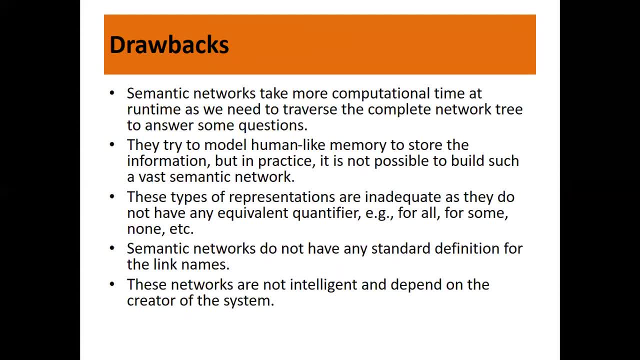 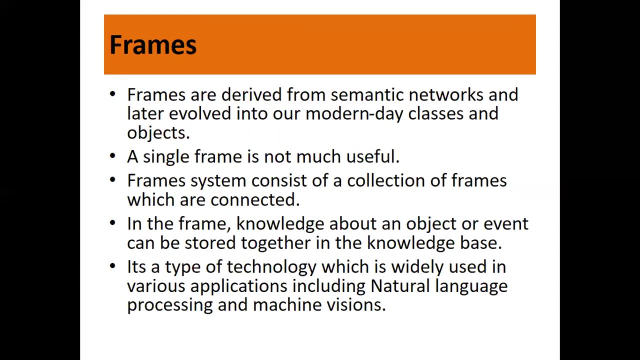 intelligent and depend on the creator of the system. no new knowledge can be created using these networks. okay, so now let us look at the another way of knowledge representation, that is, frames. now, frames are derived from the semantic networks and later evolved into our modern day classes and objects. right now, what we have, what they're using in our object-oriented programming- 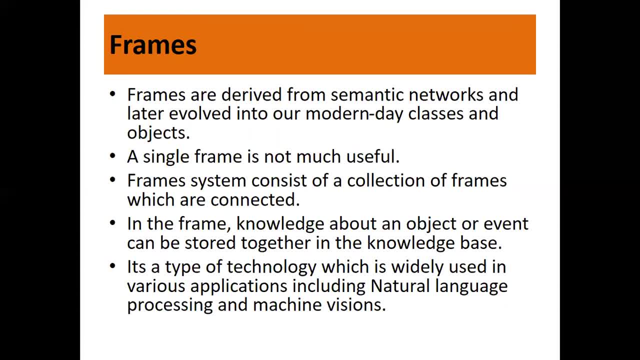 a single frame is not much useful. frame system consists of a collection of frames which are connected. in the frame, knowledge about an object or event can be stored together in the knowledge base. it's a type of technology which is widely used in various applications such as computer. 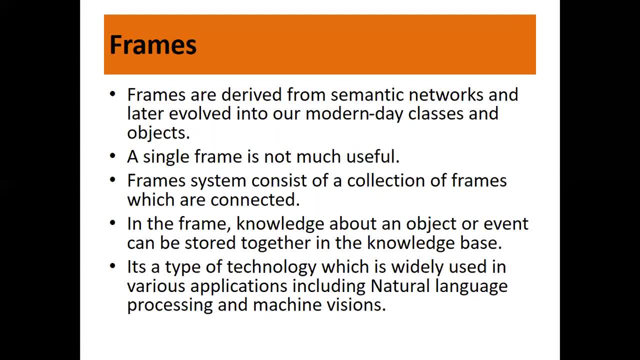 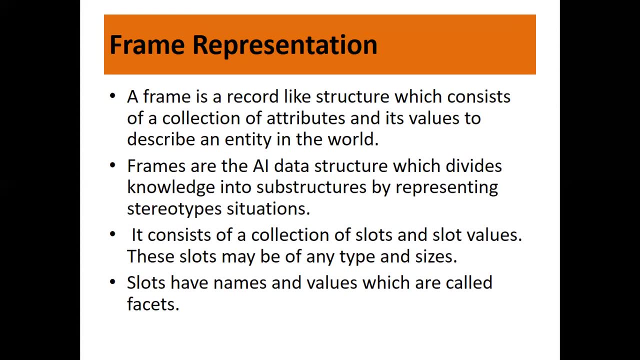 based applications, including natural language processing and machine reasons. so remember, it is nothing but again a class which can be represented using a record type structure. so how do you represent a frame? a frame is a record-like structure which consists of a collection of attributes and its values to describe an entity in the world. right, you have. 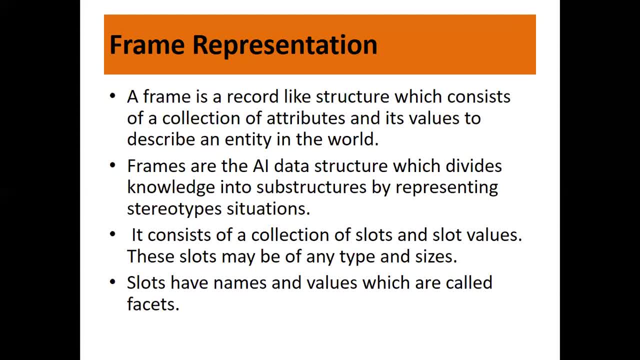 a set of attributes which describes that particular class, or then object and the values. so the frames are the ai data structure which divides knowledge into sub structures by representing stereotypes, situations. it consists of a collection of slots and slot values. these slots may be of any type and size. slots and names and values which are facets, so slots will be clear. as you see, the 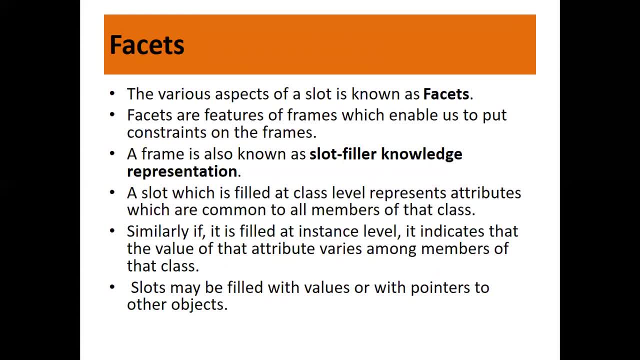 example. now, what are these facets? the various aspects of a slot is known as facets. facets are features of frames which enable us to put constraints on the frames, like what type of data can be stored. a frame is also known as slot filler. knowledge representation a slot which is filled at. 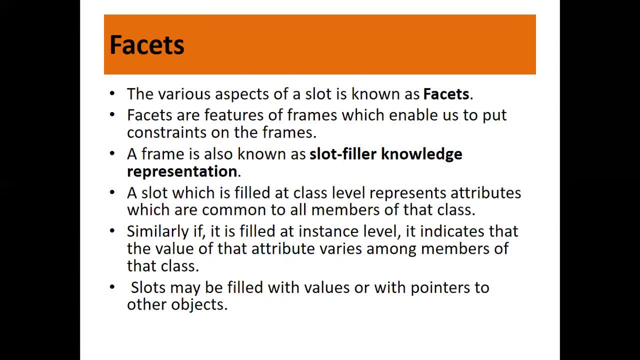 a class level represents attributes which are common to all members of that class. again, i repeat: a slot which is filled at class level represents attributes which are common to all members of that class. similarly, if it is filled at an instance level, that is, at object level, it indicates that the value of that attribute varies. 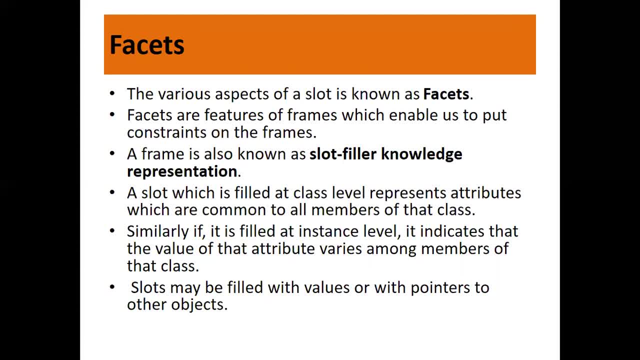 among the members of that class. that means if you have a class car and you have the instance like audi, you have instance like varna. so the attributes values of the vana and of the audi will differ, but at class level. but the attributes of class car will be same. but the instance is that the 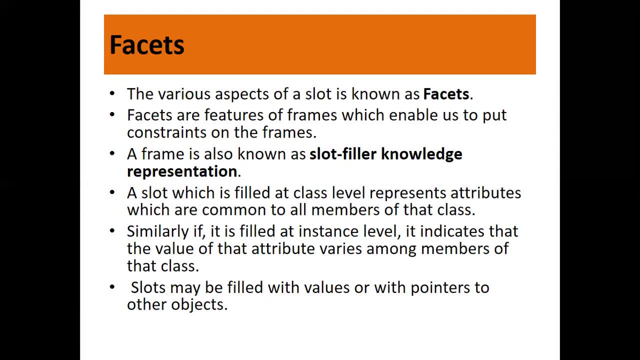 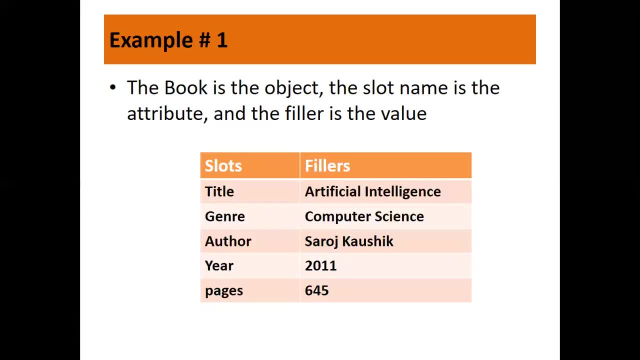 object of that class will have different values. slots may be filled with values or with pointers to other objects. right now, let us look at an example here. we are representing a book- is the object right? and we are represented using a flame. the slot name is the attribute right. the slots name: the slots are title generally. these are the 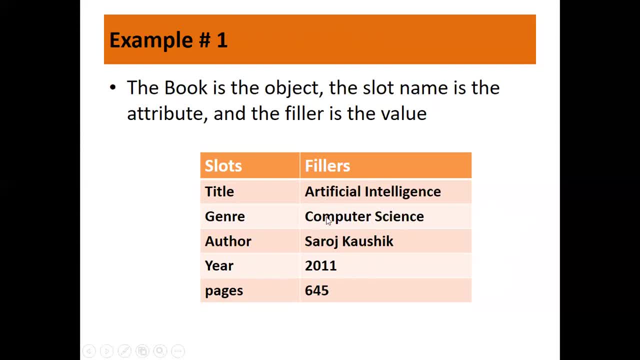 attributes and the fillers are nothing but the values of that particular attribute. now, to represent a book as a frame, what we have? we have the attributes as titles and the value. artificial intelligence, gender is nothing but the computer science. the attribute is author and the value of 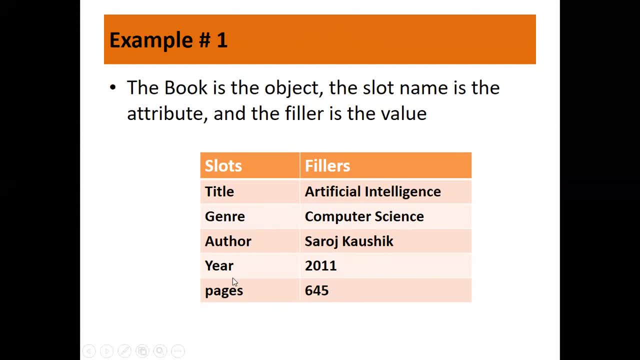 the attribute is saroj kaushik. the year 2011. pages 645. now, in this whole thing, you can get the whole data about a book right, but it's not a class book. it is an object of class. you, similarly, you can have a frame for a class book and this is for an object book. let us look at: 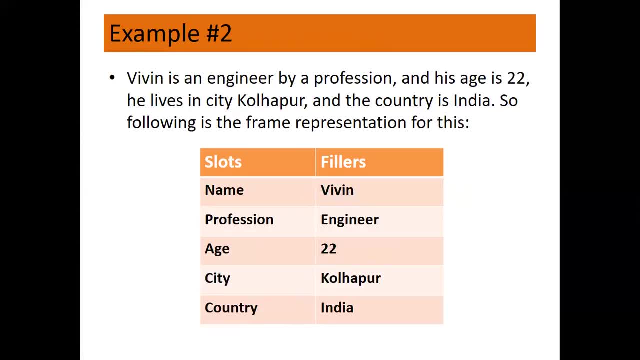 another example where the statement is given and how do you represent it using a frame. now, the statement is: what women is an engineer by profession and his age is 22. he lives in city, kolapur, and the country is india. so how do we represent it? again, your slots and the fillers. 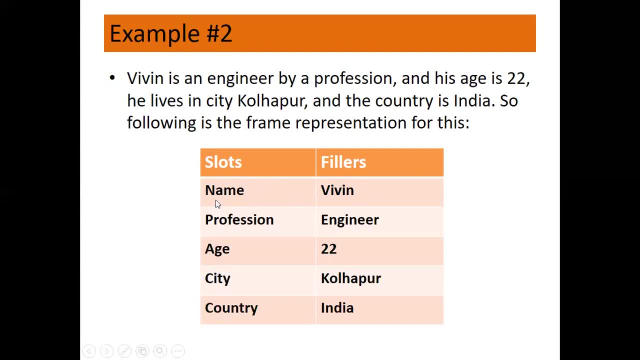 now, what are the attributes of a person? name, profession, age, city, country. now the data is given here. just put it: name: women. profession: engineer. age 22. city he lives in kolapur. country is india. now this whole thing gives you the. this whole statement can be represented using this single table, which 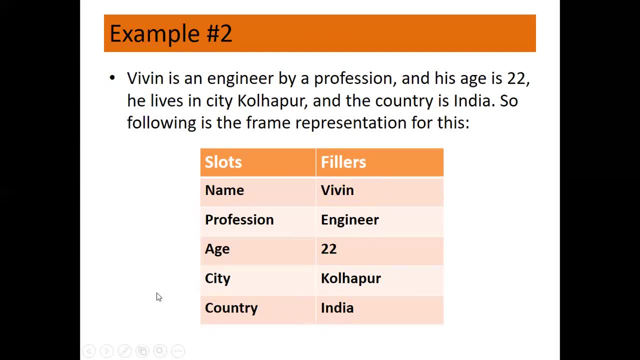 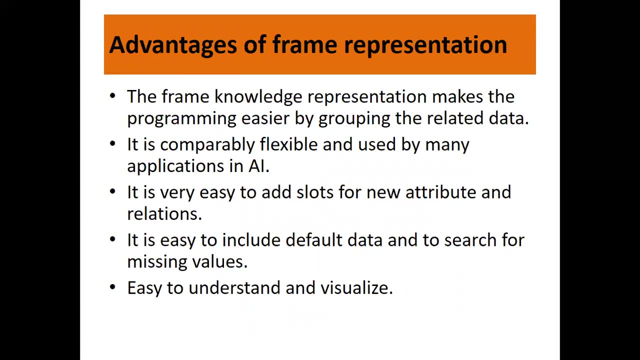 is nothing but a frame. i hope the concept is clear now. what are the advantages of frame representation? the frame representation makes the programming easier by grouping the related data. now looking at it, it must be very clear now how we represent the objects in a object oriented programming. it's 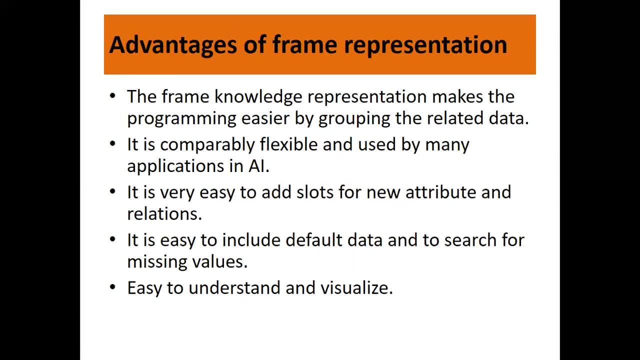 comparably flexible and used by many applications in ai. it is very easy to add slots for new attributes and relations, right, so slots is nothing but the attributes, what we're adding. it is easy to include default data and to search for missing values, and also easy to understand. 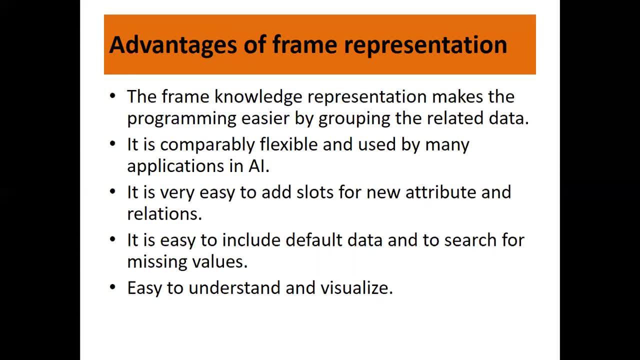 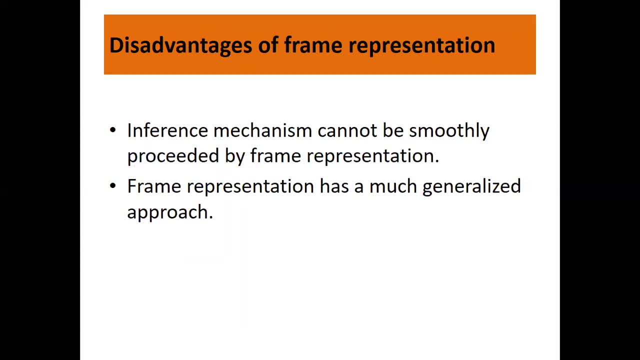 and visualize. let us look at the drawbacks. so what are the disadvantages? inference mechanism cannot be proceeded by frame representation. now what is important? inference? inference is what- getting going through the knowledge base and coming out, coming up with a new knowledge using the existing knowledge base. so it is very difficult. inference mean deducting the knowledge.